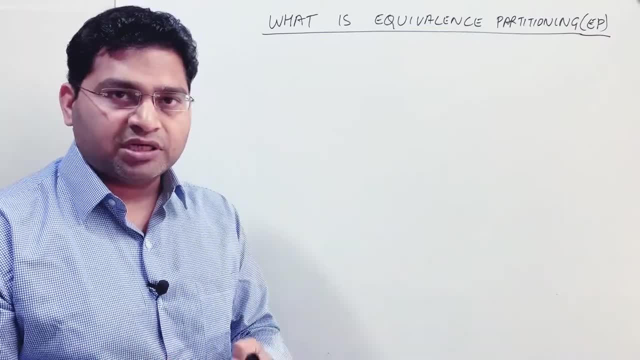 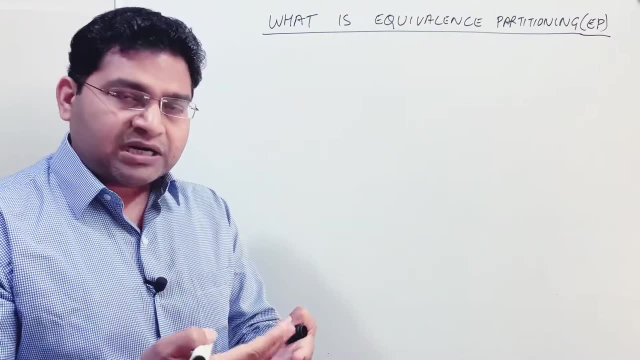 watching this particular video, would have definitely bought something or the other from the online store. and there are sales going on most of the time and sales are, you know, divided into different categories. Say, for example, you spend $100, you get 5%. you spend. 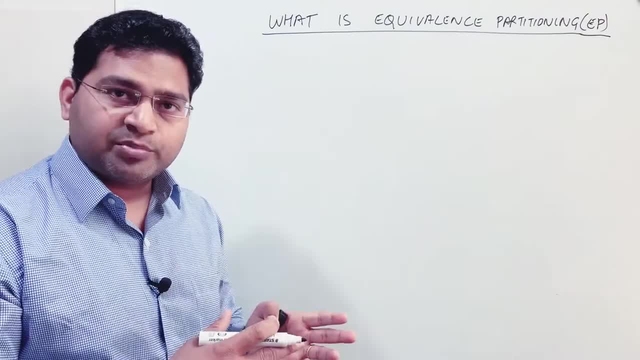 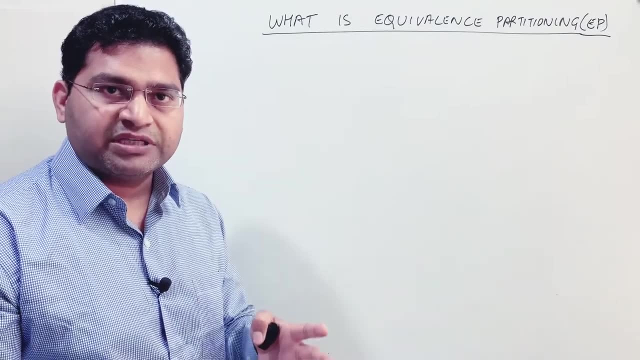 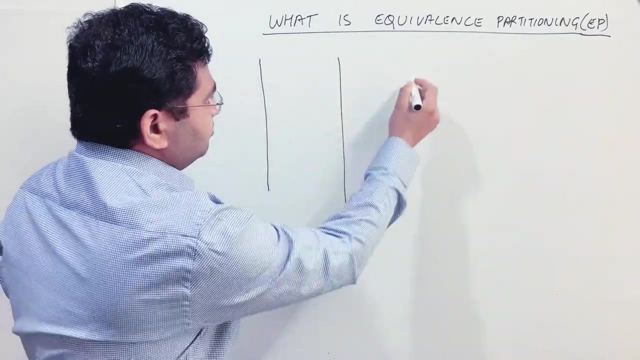 $1 and above up to $200, you get another percentage of discount right. Say, for example, you are going to test that particular discount module in the software in the e-commerce portal. So how we can have these partitions right. So let's first divide the partitions, okay. 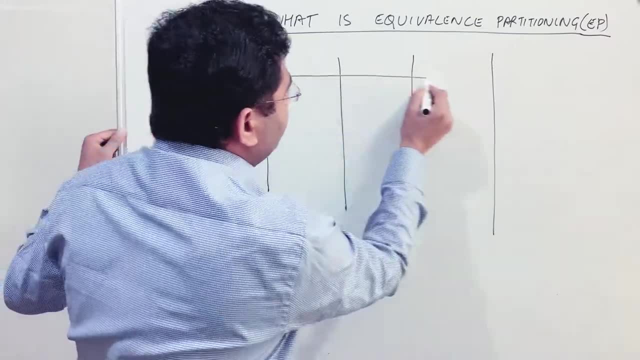 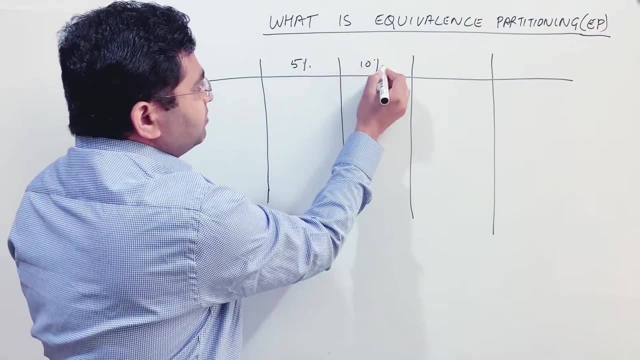 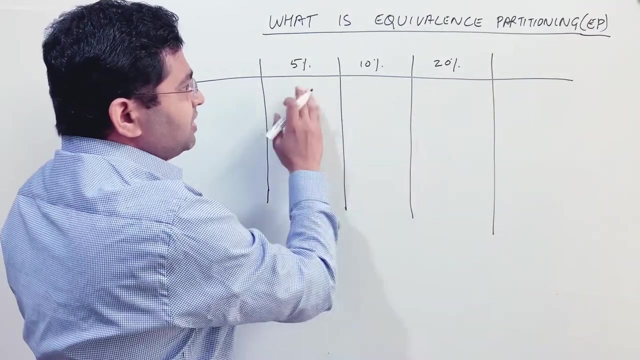 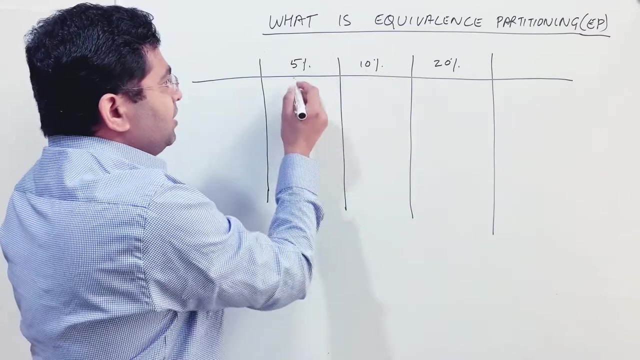 Now say, for example, there is a e-commerce portal and that portal has three different tiers of discount. Okay, 10% and 20%. So these are three different discounts that you have available on a particular sale that is going on in the e-commerce portal. Now 5% discount is applicable for any customer. 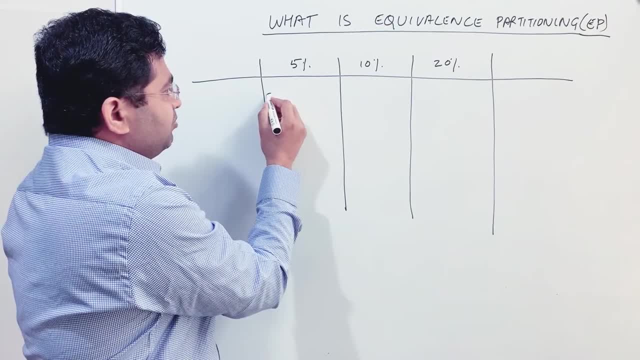 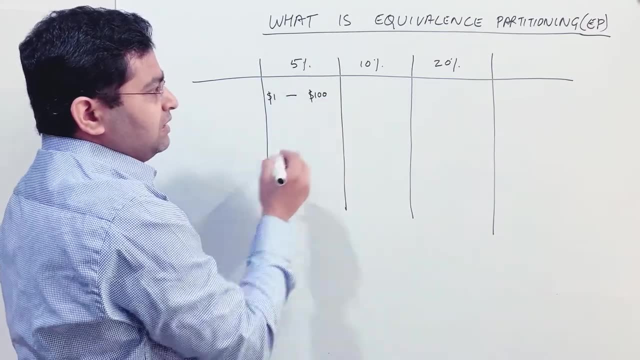 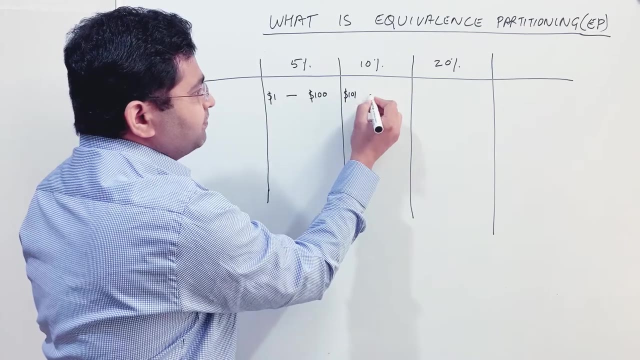 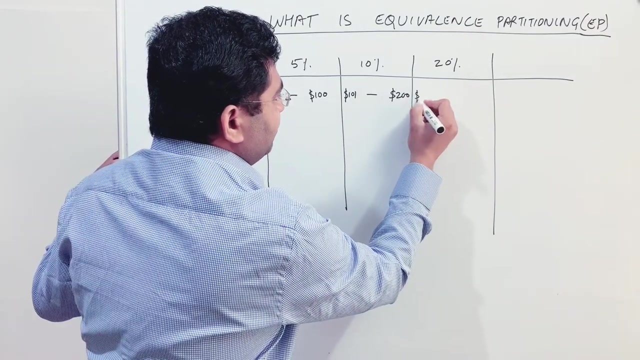 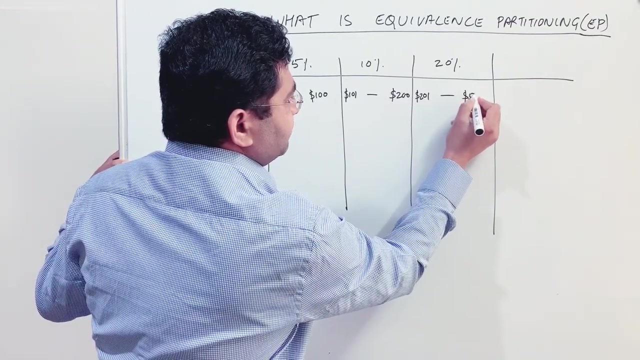 who is making purchase of, say, for example, $1 and up to $100, okay. Then 10% discount is applicable to a person who is buying from $101 up to $200, okay. Then 20% discount is applicable for a person who purchases from, you know, $200 to $500, okay. So 1 to 100, 101 to 200, 201 to 500, applicable discount is 20% discount. Okay. so what about 400 dollars before that 100 to 200, do we agree with the saying? Okay, then 50% discount is fine for any customer who is not using Google Play Maker already. You can also look at the� сод big site and you can also do a release code adress for that. okay, There is a one-shot解 into applying for a Thatsugord in which it says the speciallocal discount code from a qualified consulting. 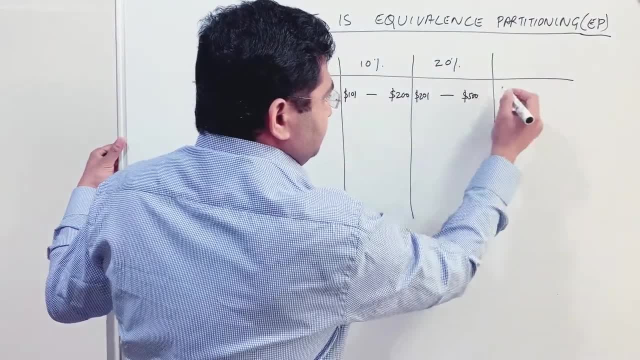 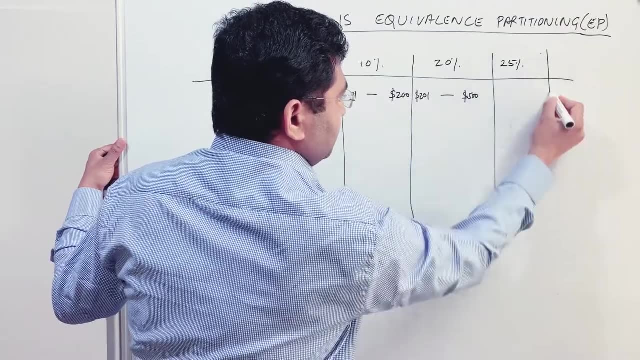 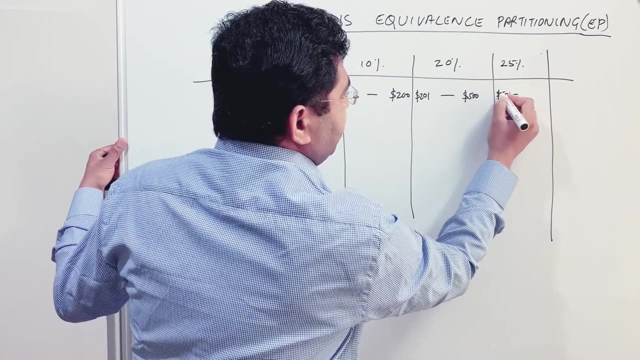 Is that feasible? and then anything above 500, say for example, is 25% discount. let's have one more partition there, okay. so anything above 500, so which is 501, and up to the max value allowed on the portal, right? so, for example, max value will see max value. 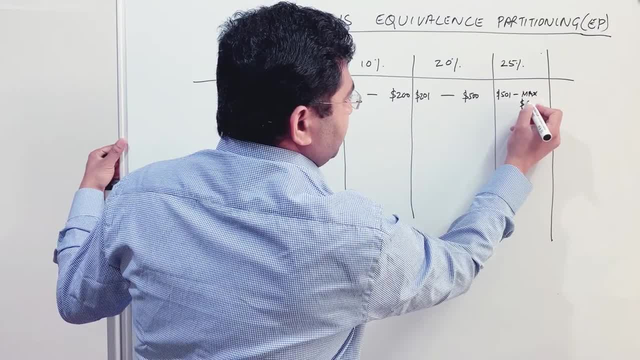 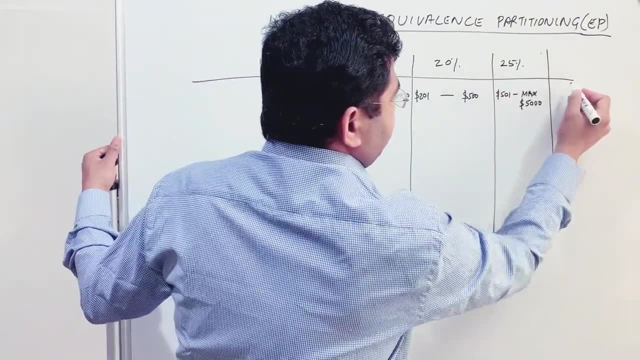 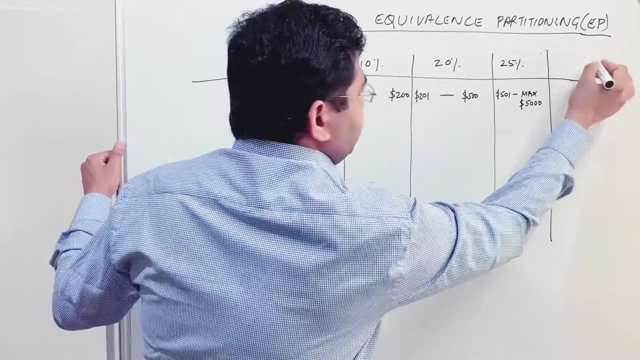 allowed max purchase value allowed is, say, for example, 5,000. okay, so up to 5,000 the discount will be 25%, and after 5,000 there shouldn't be any purchase allowed. okay, so we'll we'll write these later and this one later. so now, if we talk, 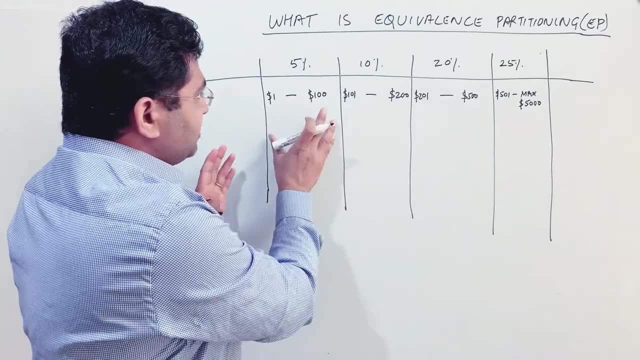 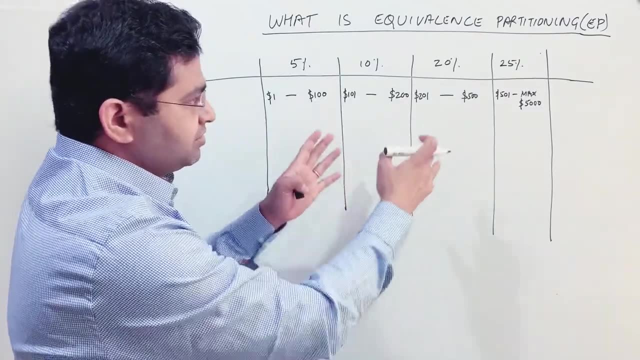 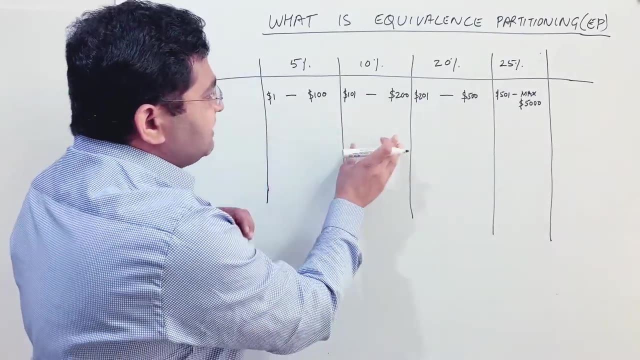 about the equivalence partitioning. if we see that we have divided these discount percentage on an e-commerce portal into different partitions, right, and when we talk about equivalence partitioning, the partitions are five percent, 10 percent, 20 percent and twenty-five percent are considered equal. so if you pick any value in this, 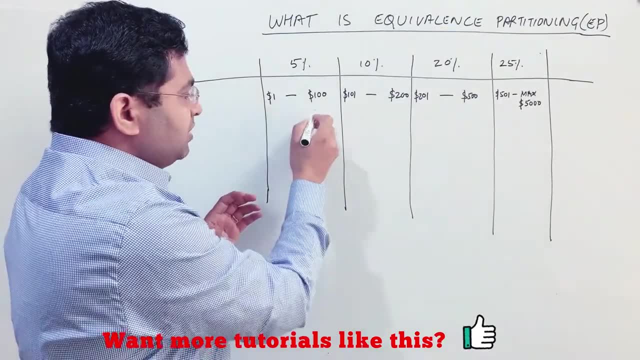 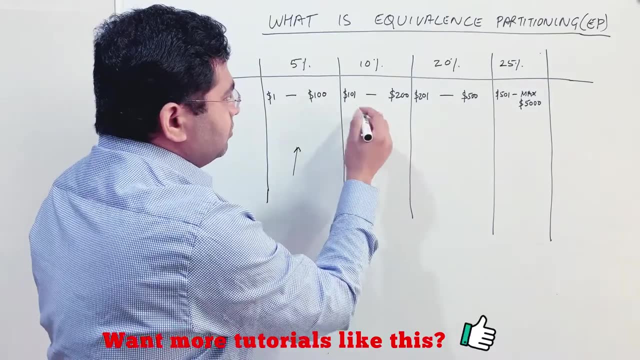 partition. any purchase value from 1 to 100, it will be considered same and 5% discount will be applied. if you pick any other value from 101 to 200 dollars, 10 percent discount for ALB or 90 percent will be applied if you瑞 have a. 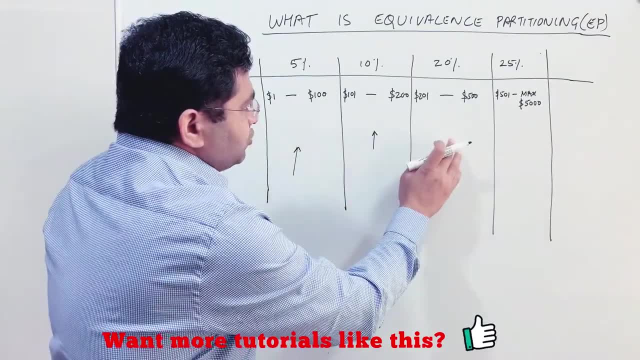 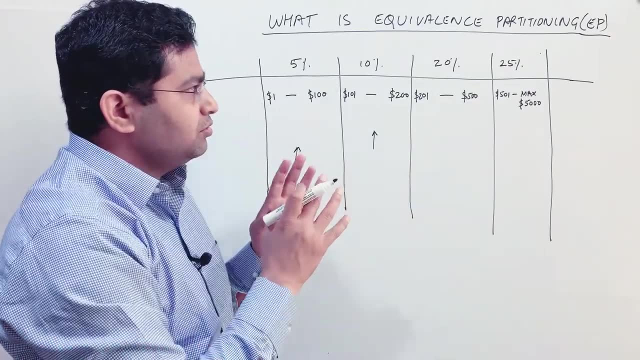 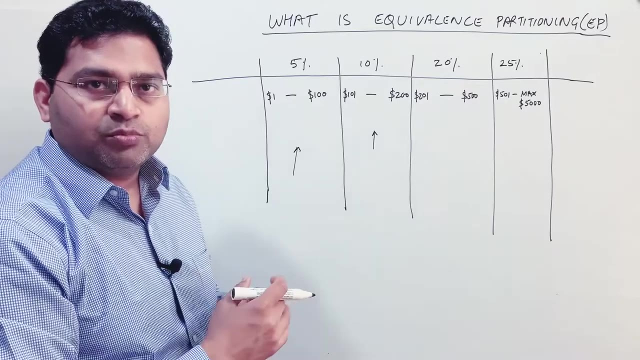 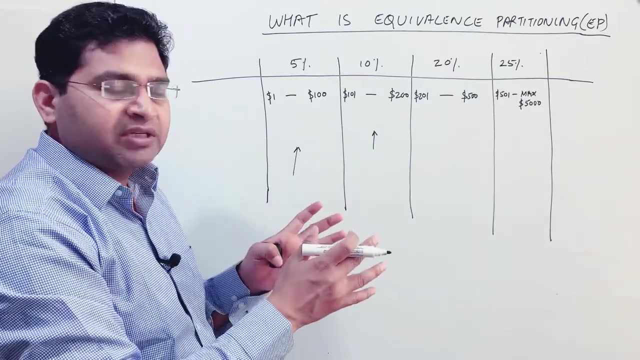 should be applied right. similarly, 25, 20 percent and 25 percent. so when we divide the you know module which accepts certain values and, based on the values, certain outcome needs to be applied, then those sort of module, or dividing those module in equivalence partitions is known as equivalence partitioning. okay, 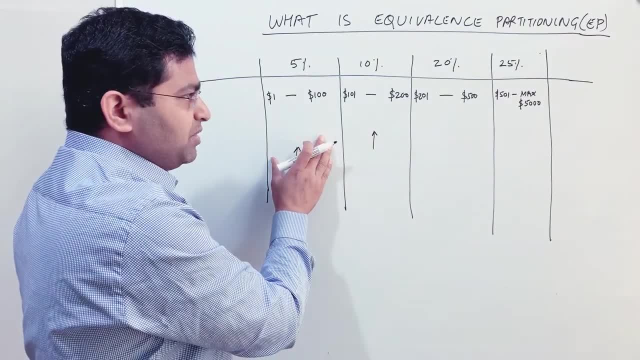 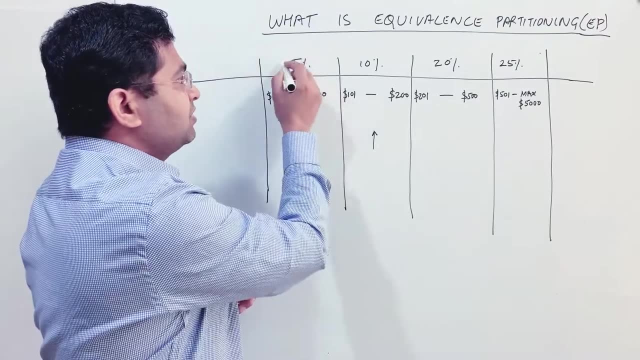 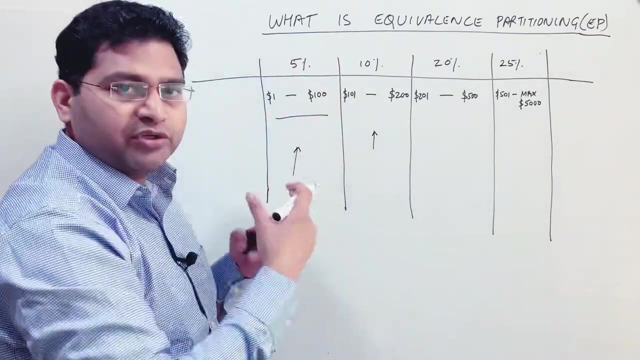 so in this case, the discount module of the application accepts the dollar amount of the purchase amount and, based on those dollar and purchase amount, you get the different discounts. okay, so this is basically your input and this is the basic output that you want to verify, right? if I have this, if I have the you 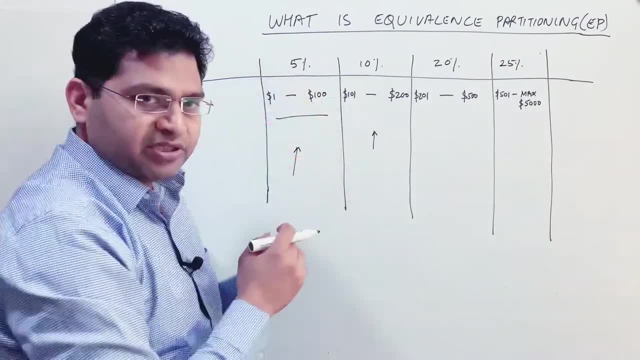 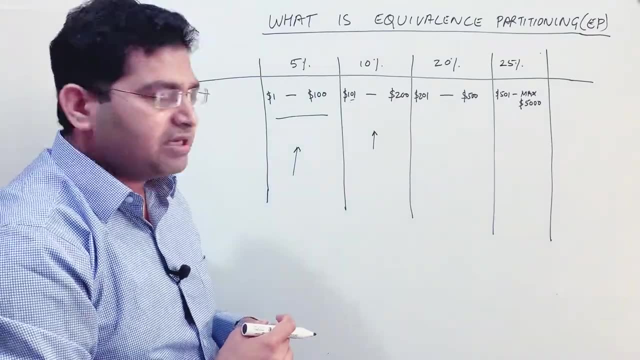 know items in card which are $100, then I should be getting 5% discount. if I have items in cart and I have completed the purchase of hundred and one dollar, I should be getting 10% discount, right? so this is what partitioning is. so we have. 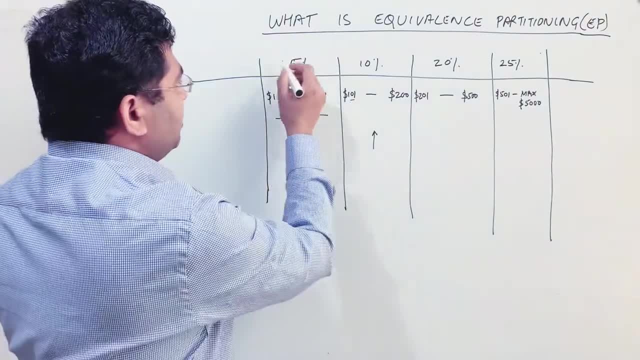 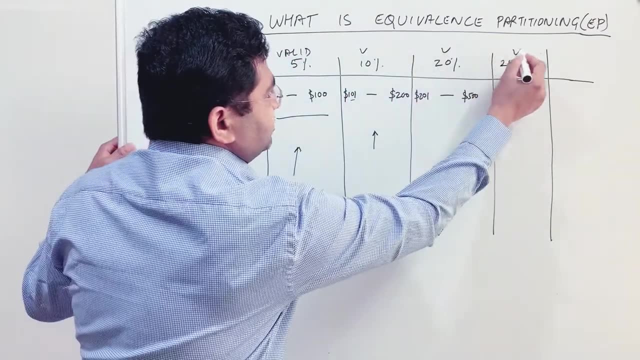 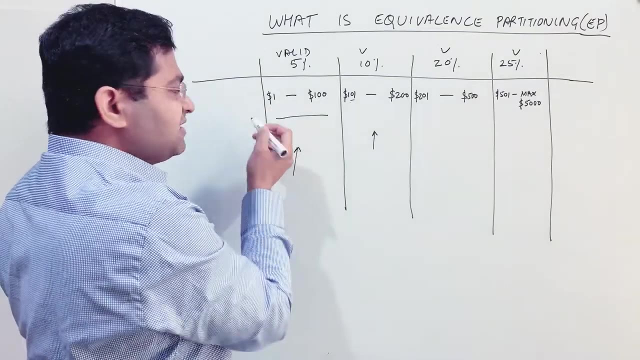 divided the module into different partitions. now these, if we consider, are the valid partition. right. so this is valid, this is valid, this is valid and this is valid. now, what happens for the purchase which is less than one dollar, say, for example, 0.99 cent? should this be allowed on the? 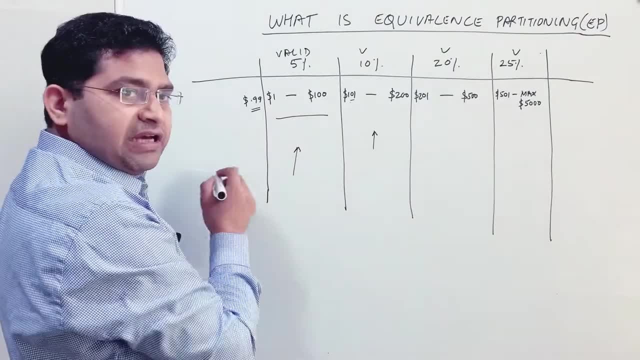 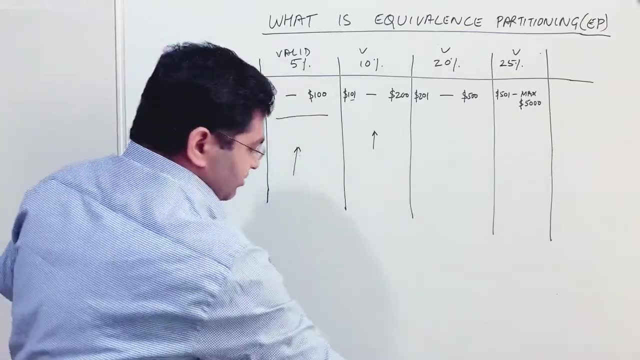 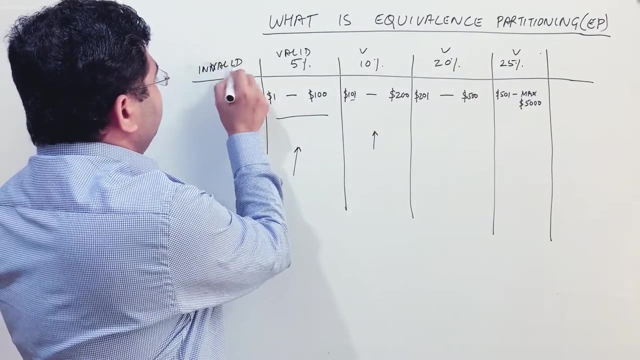 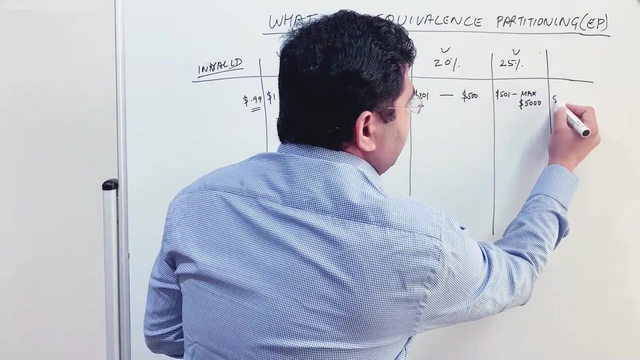 application, right. so if this shouldn't be allowed in the application or this purchase shouldn't be allowed, then in that case what you do is: this is invalid partition, okay, so this becomes in valid partition. and here because the max purchase amount is five thousand, so I shouldn't be allowed, or as a customer, a. 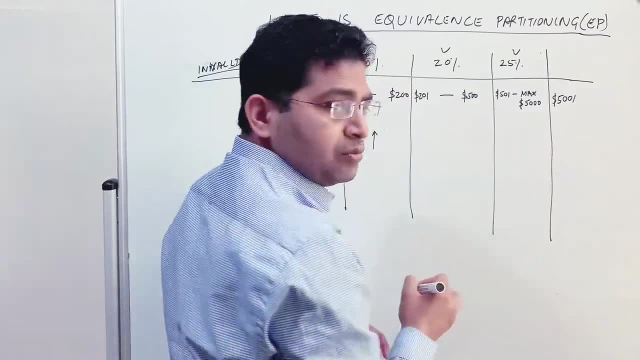 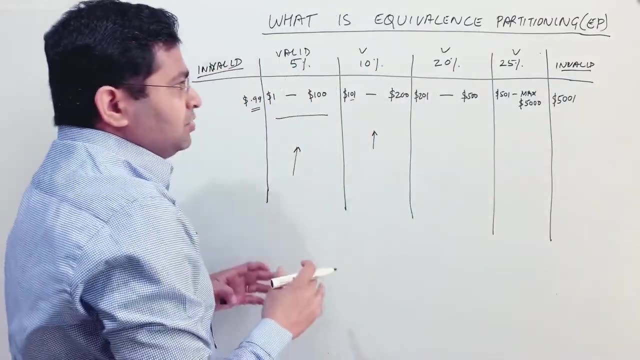 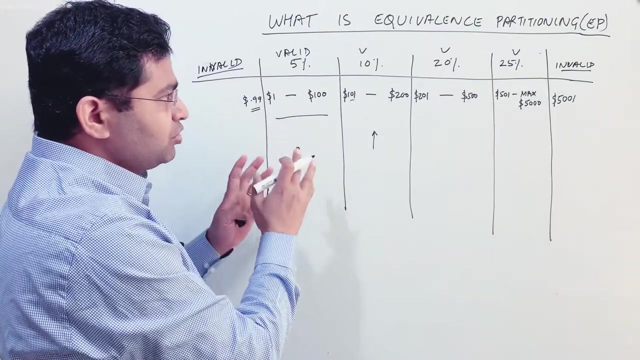 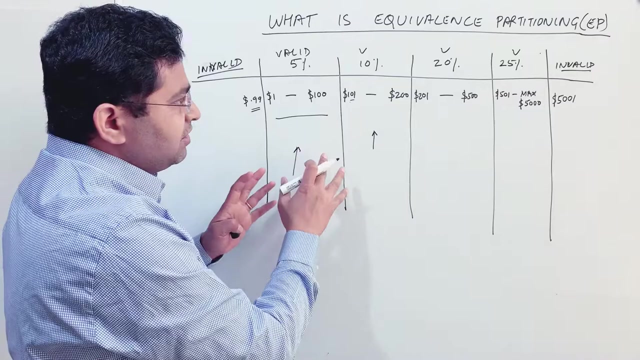 customer shouldn't be allowed to make a purchase of five thousand one dollar, so that's another in valid partition. okay, so now you can see that the module of a discount. once we have divided that module into logical valid and invalid partitions, we are now having a clear understanding of when the partition or 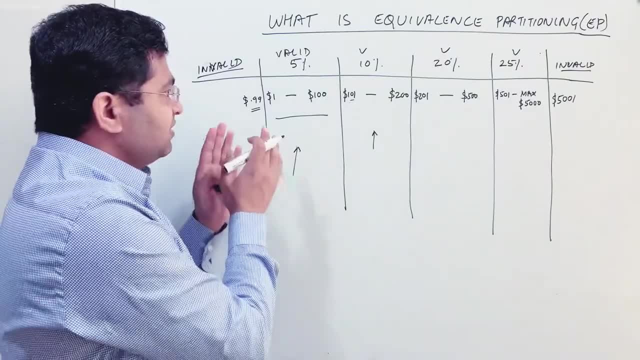 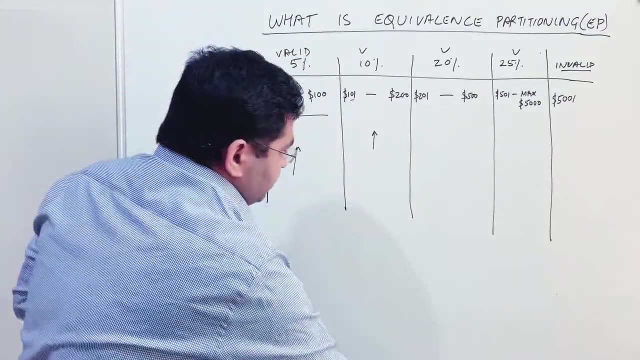 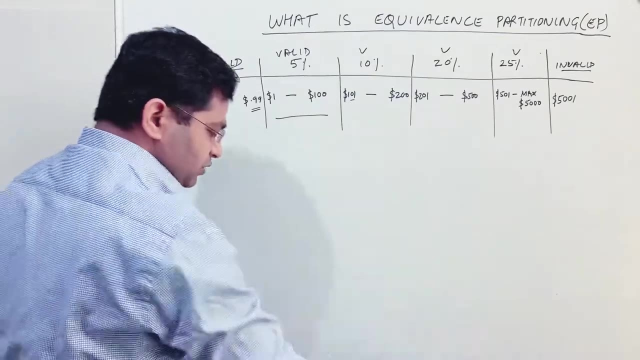 what values we need to provide or what values we need to test with to get different discounts right. so this is very important to understand in order to get the best number of test cases, or minimum number of test cases, which will give you the best coverage. okay, so now we don't have to do the random testing. 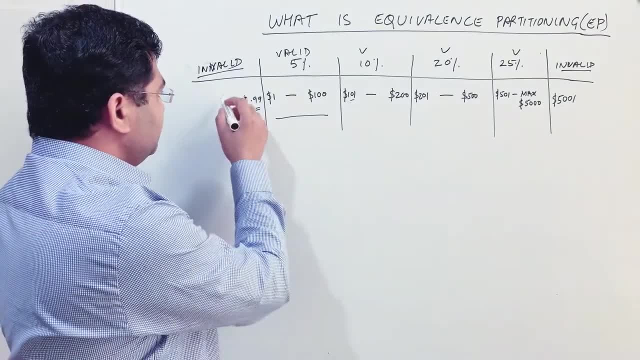 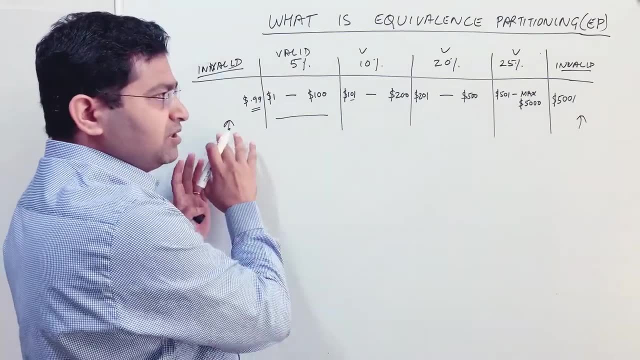 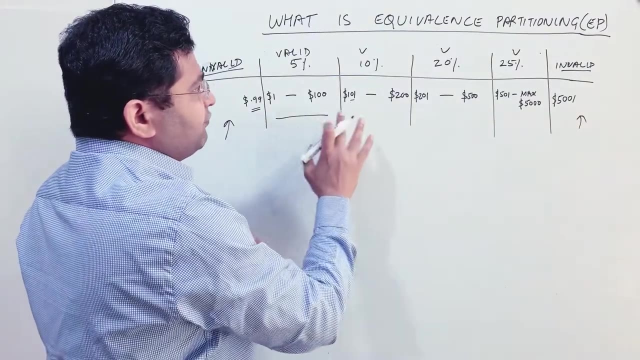 in this particular case, what we can do is we can test, you know, invalid partition at the lower end, invalid partition at the higher end, with some of the values in the invalid partition and value in that particular case. remember you know higher and invalid partition. then we can test with some of the values. 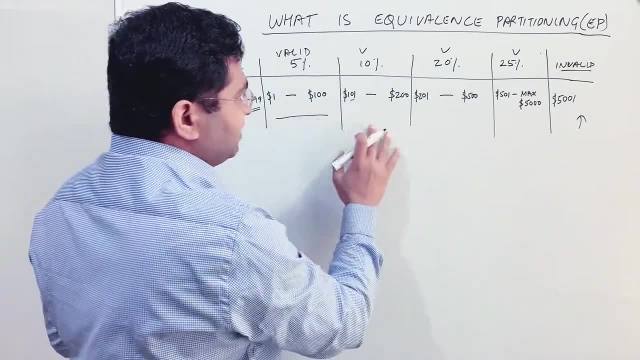 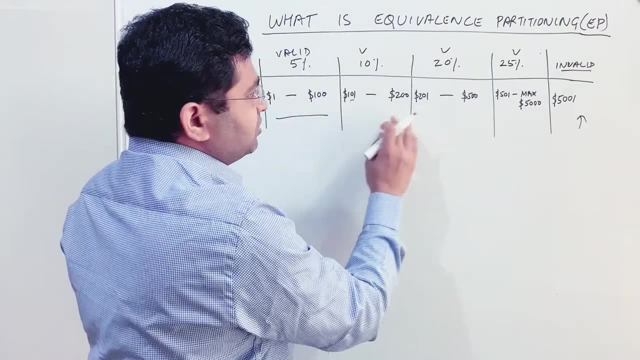 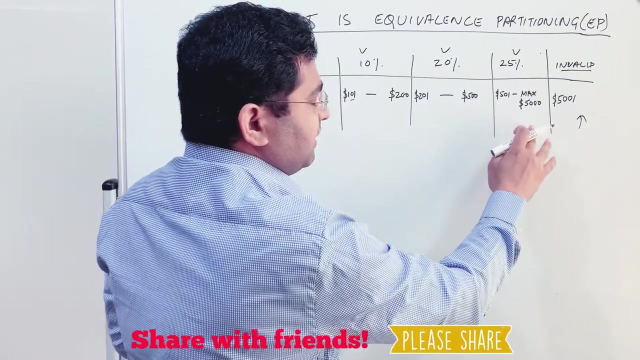 in the valid partitions, right in each of the valid partition, we can pick. say, for example, here we'll pick $50, $100, here we'll pick couple of other values, here we'll pick 201, you know 499, 300, and here we'll pick, say, for example, 501 and you 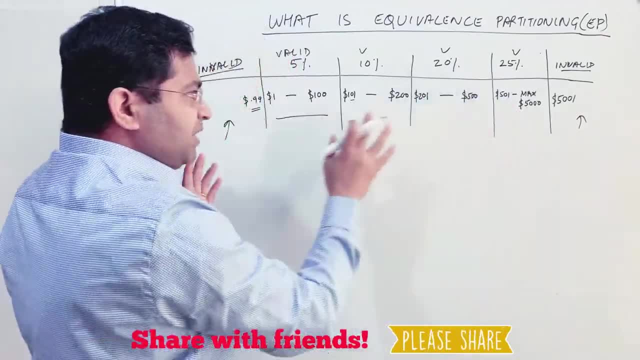 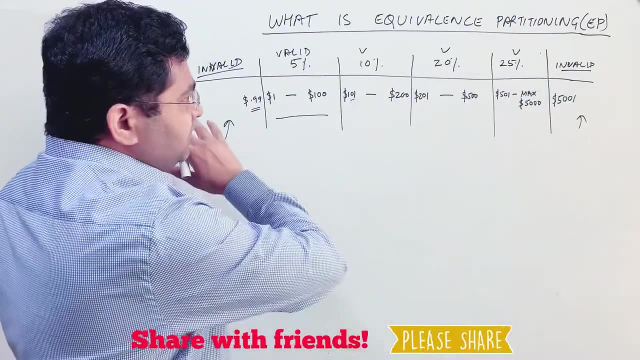 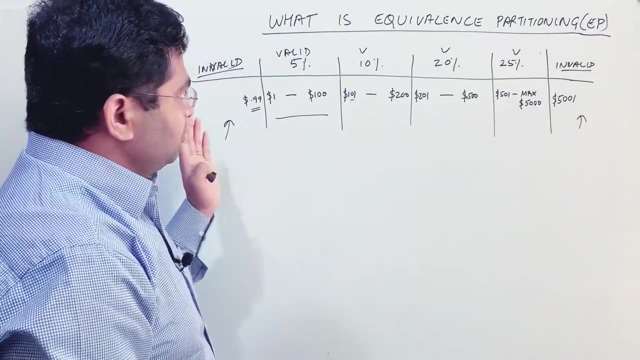 know four thousand, five hundred or five thousand. so if we pick couple of values from each of these valid and invalid partition, we are getting good coverage and we are testing each of these partitions of the discount module of e-commerce application right. so this is what equivalence partitioning is you? 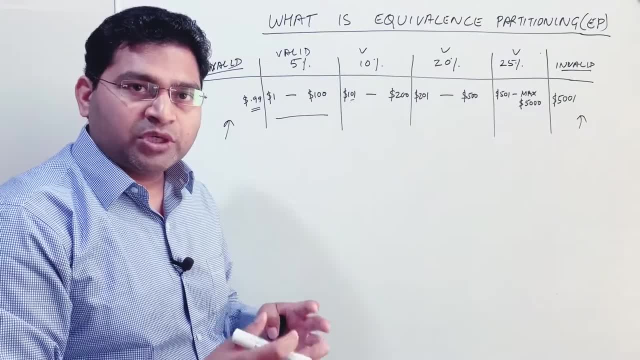 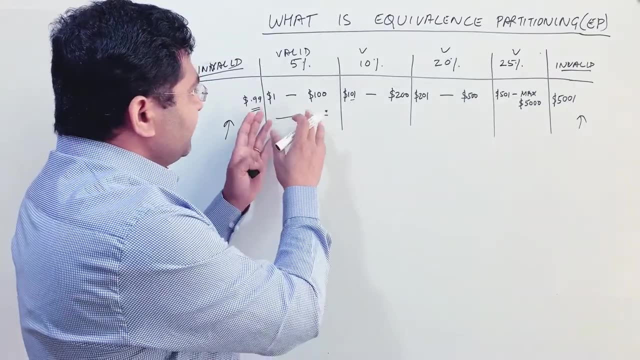 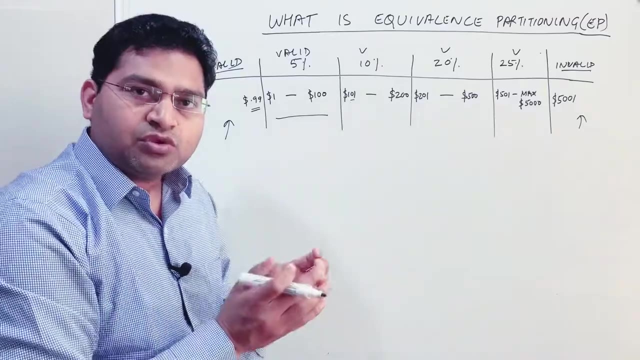 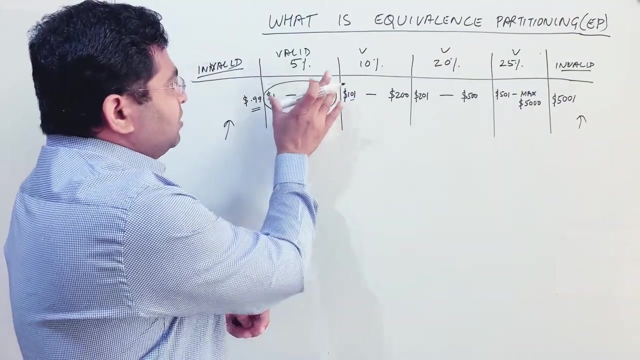 divide the module of the software which behaves, you know equally or logically equal in certain scenarios. so you divide those into you know valid and invalid partitions and then within those partitions, it doesn't matter what values you put within those partitions. if they are within that range, the output should still be considered similar and should 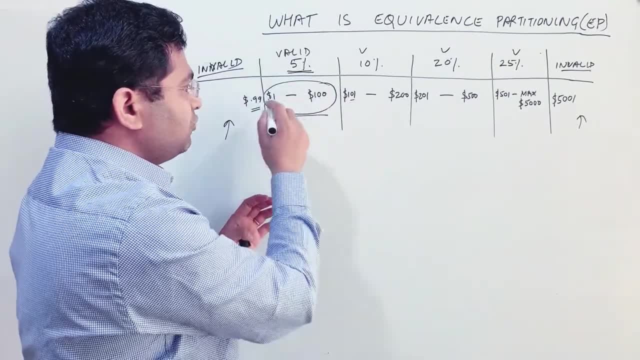 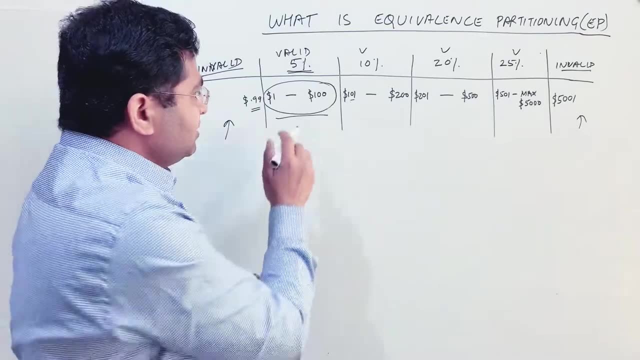 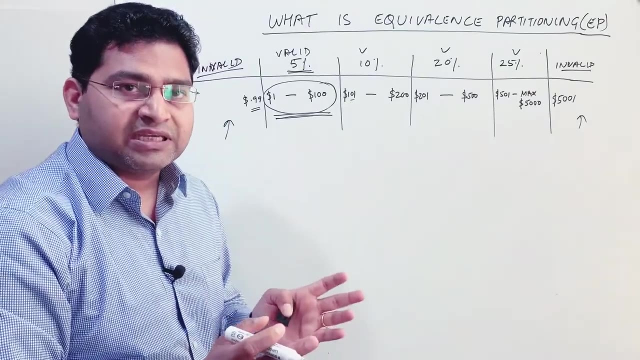 be same. so in this case it doesn't matter what values you know you put from one, two hundred should still be considered as five percent discount, right? so this is, you know, logical partition that we do in software testing to minimize the number of cases that you are going to test against. now you can't keep testing. you know purchases from one to. 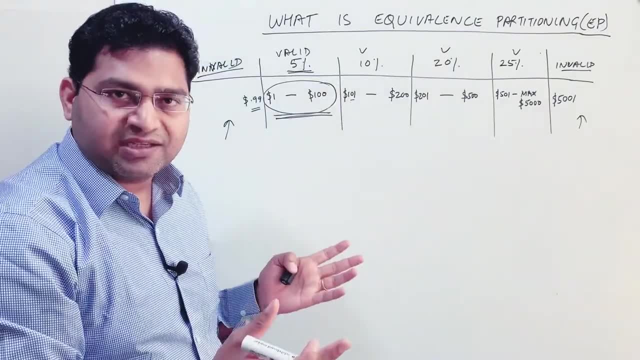 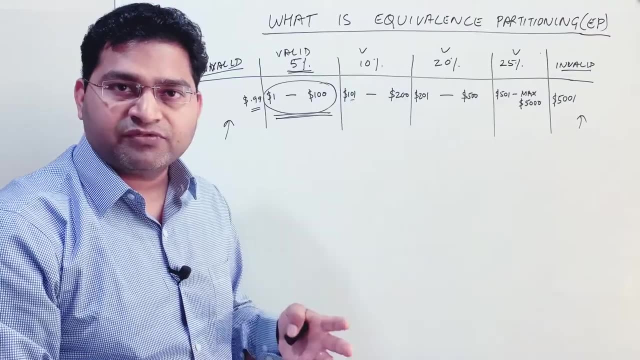 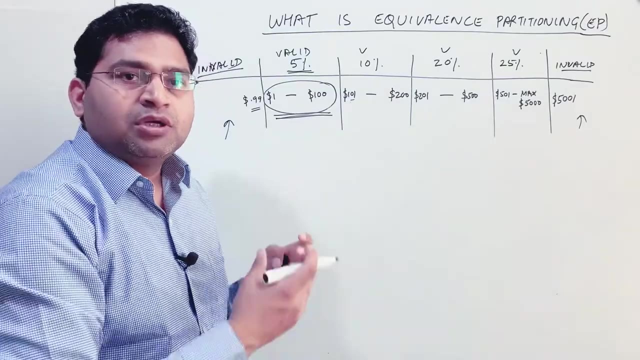 hundred dollars. so there will be no like hundred test cases all alone to test this five percent discount. and we have understood in the software testing principle that exhaustive testing is not possible and that is why these are the techniques. equivalence partition is the technique to come up with minimal number of test cases which will give you- which will still give you- a very 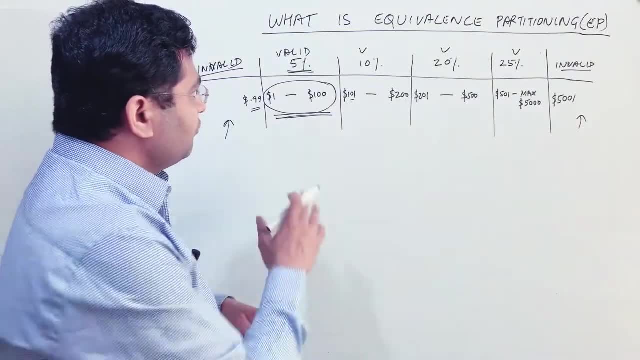 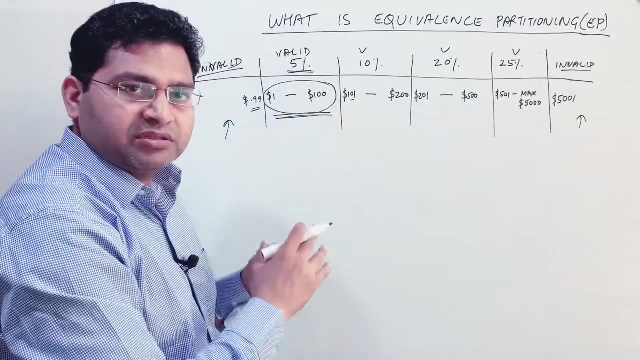 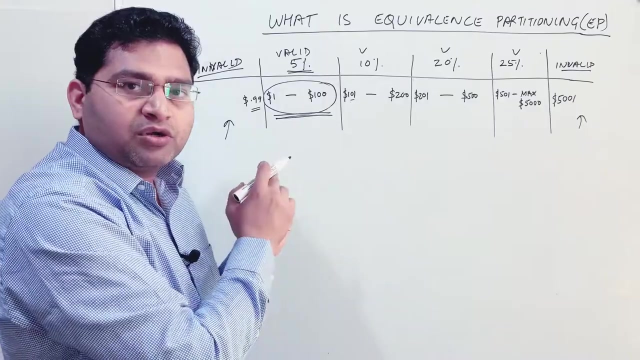 broad test coverage because logically the software will consider all the values within these partition as same. it will take them as same. it doesn't matter you put all hundred values or you just just pick higher and lower and one or one or couple of middle values and test it now: equivalence. 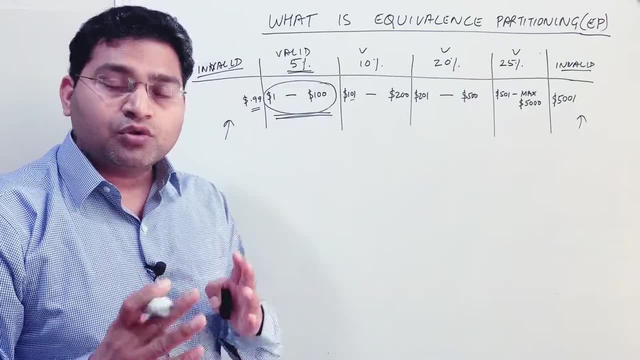 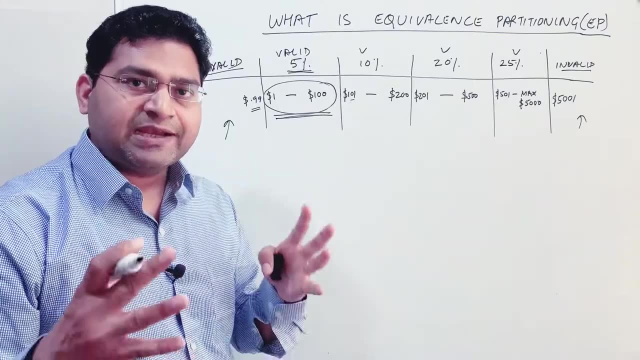 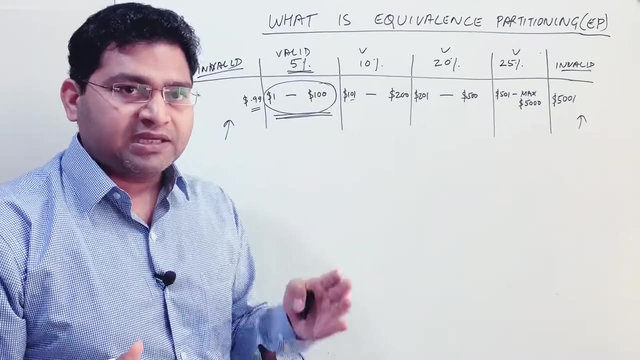 partitioning doesn't go you alone. it goes together with boundary value analysis, which i'll cover in the next tutorial, and when we, when ep and bva both go hand in hand, that brings a lot of strength to documenting your test case and you will be, you know, coming up with scenarios that will help you to get. 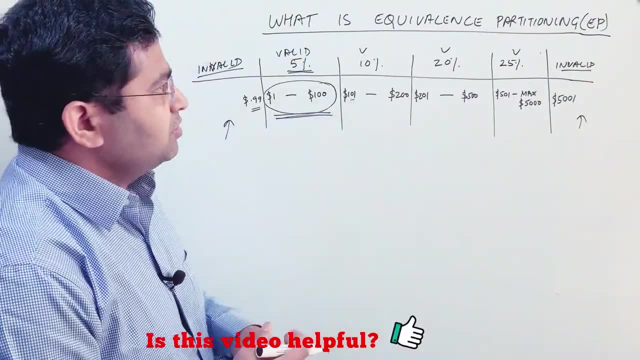 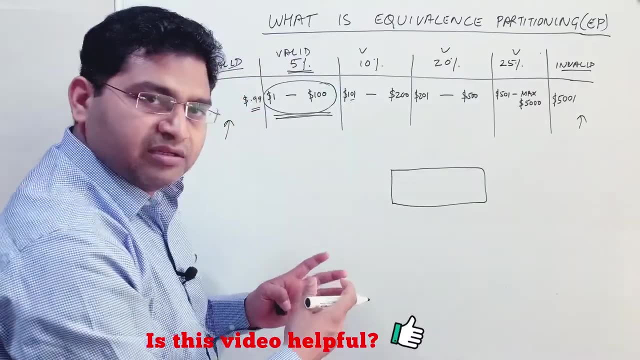 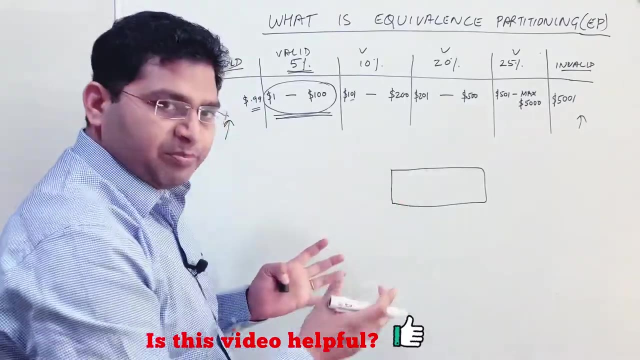 the best coverage. okay, so this is the discount example. now let's take an example of you know example of the page which has the input box right. this would this could be you know example. an interviewer might ask you say, for example, there is a web page and on the web page there is a text. 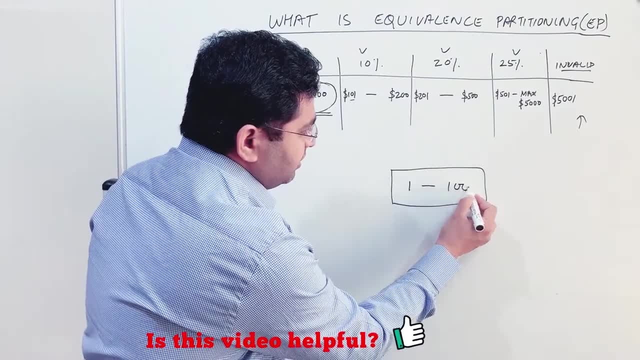 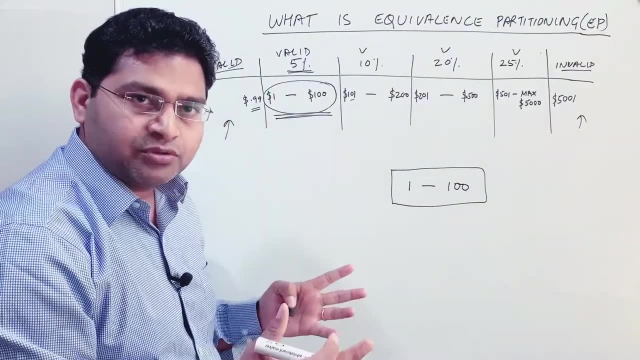 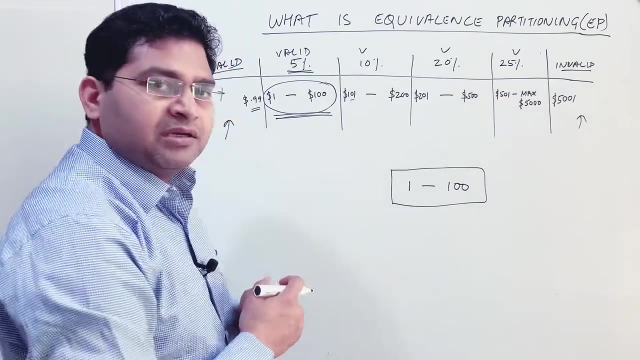 box which accepts the values from 1 200. okay, and only whole numbers are accepted. so if this is the example, interviewer comes and asks you to get me the equivalence partition for this particular scenario. okay, so how you can get the equivalence partition in this case you. 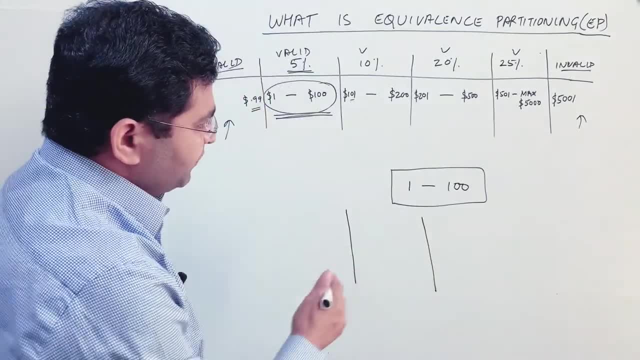 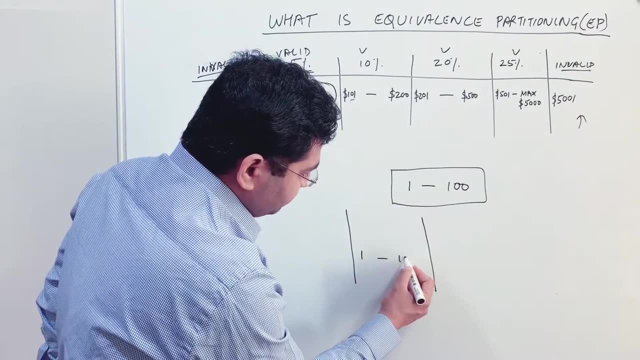 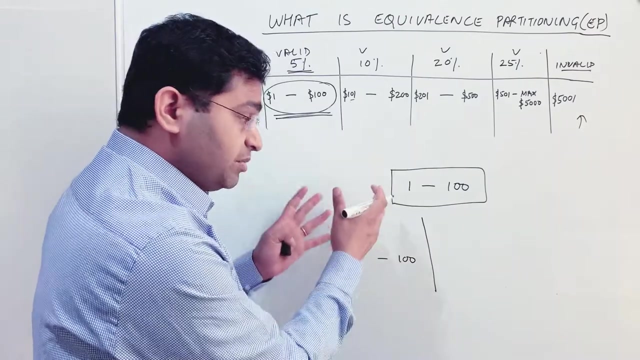 can simply have this. so this is the text box. it accepts the value from 1 to 100. so you can say: 1 to 100. okay, this, these are the values. so anything between 1 to 100 are the values that should be accepted. you should be able to submit so. 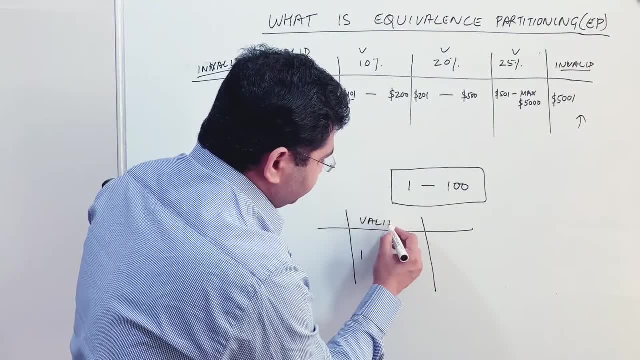 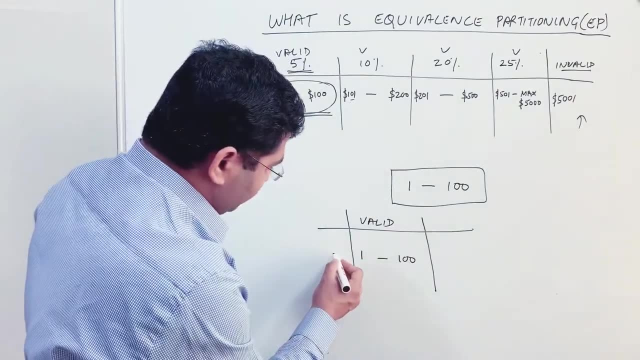 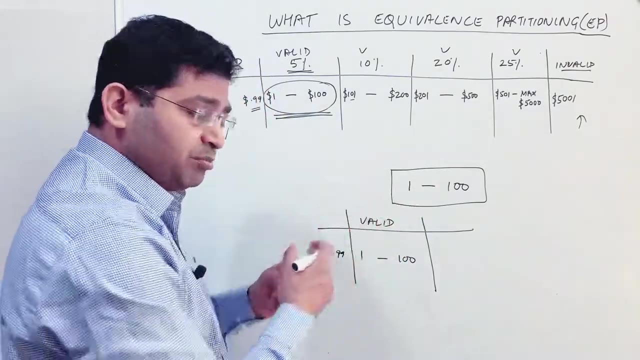 you can say this is a valid partition, okay, and then anything less than 100, okay. so you can say 0.99. you can ask question that clarify that this text box accepts only whole numbers, okay, so in this particular case, if it accepts only whole numbers, so it shouldn't accept any decimal values, right? so anything less. 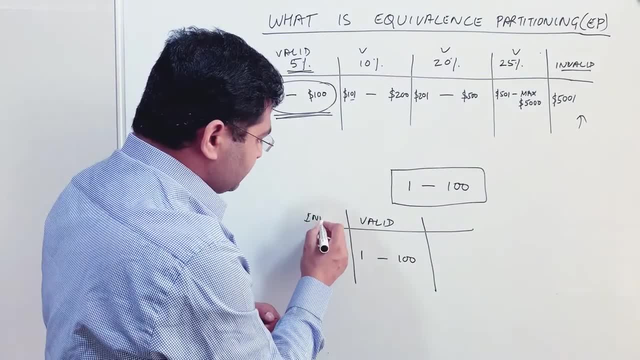 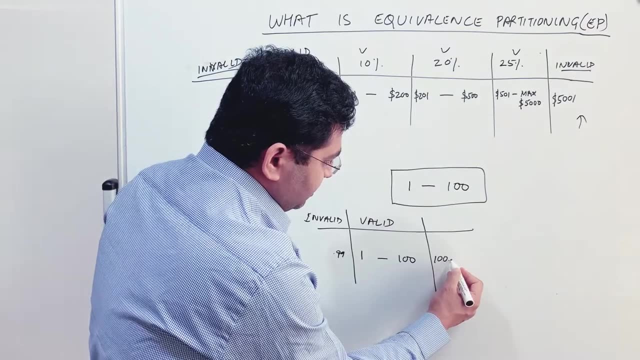 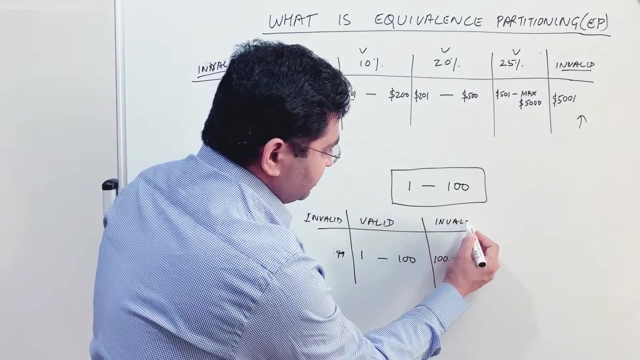 than 1, which is 0.99, should be considered as invalid partition. okay, and anything above 100, say for example, hundred point zero one, if it is a decimal value, should be considered as invalid partition as well. okay, so in this particular case, we have come up with three partitions, so you'll be you. 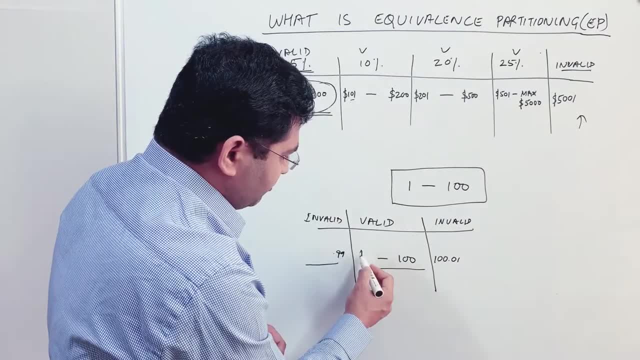 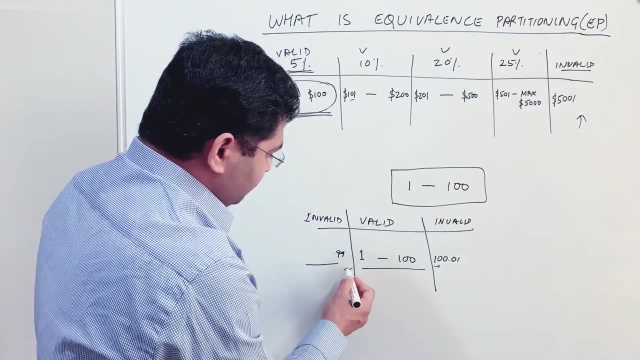 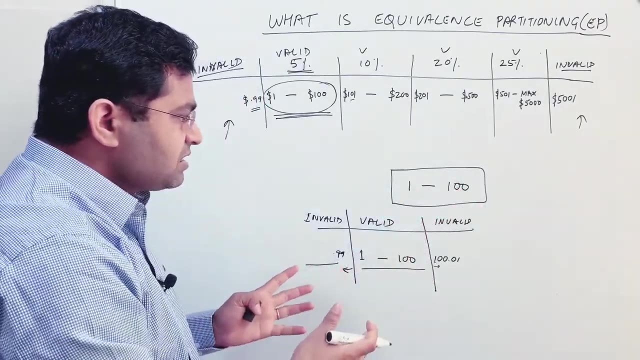 know having a partition, a valid partition, which will accept the value between 1 to 100, including 101, and invalid partition- anything above 100. anything less than 1 will be considered as invalid partition, right? so if this is something which is being asked, this is how you can explain to the interviewer and can you know? 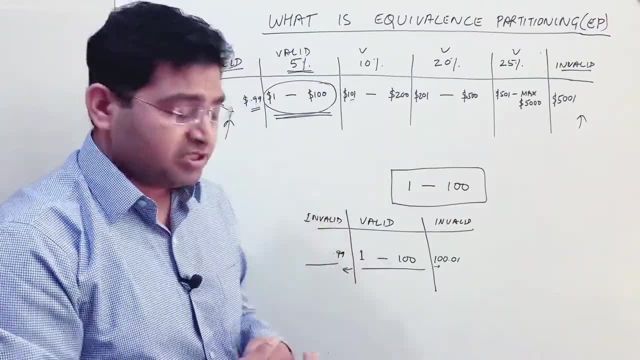 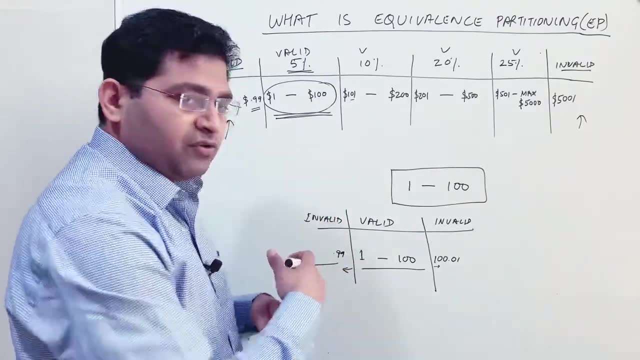 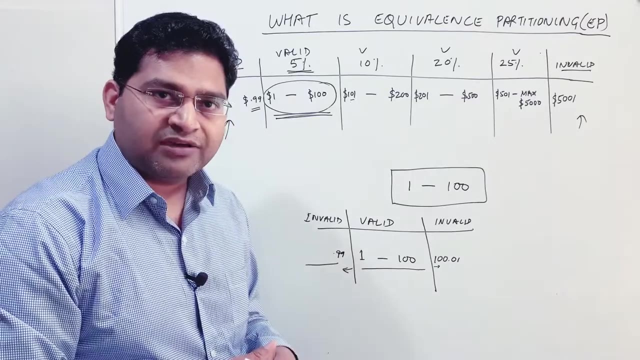 definitely show that you know all these concepts, because these concepts you will be applying day in, day out in software testing, so very important to understand. and you can think of a lot other examples and if you want to get me you know, answer any of the doubts that you have or examples that you have for a girl.